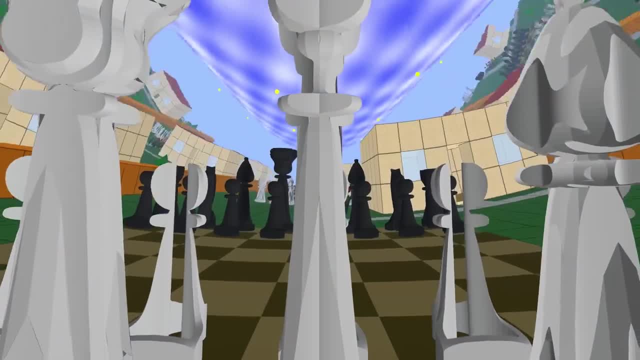 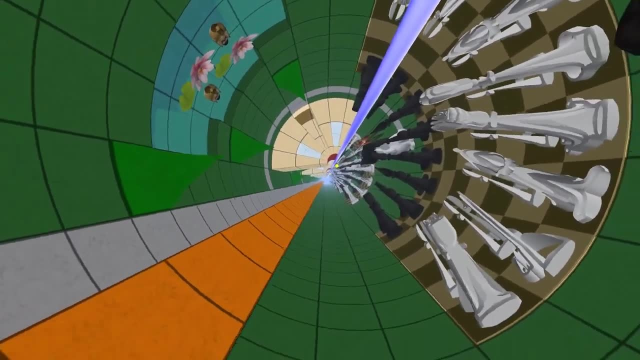 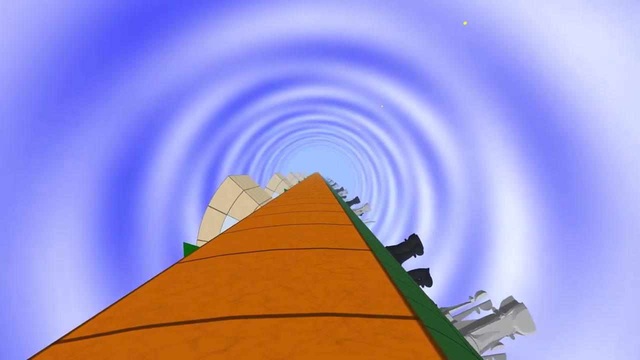 But maybe it's not the world that repeats, but the world is simply wrapped in a sequence. Now the game is played on the inside of the cylinder. We could also imagine it to be played on the outside. Now you might have noticed that our world repeats not only horizontally. 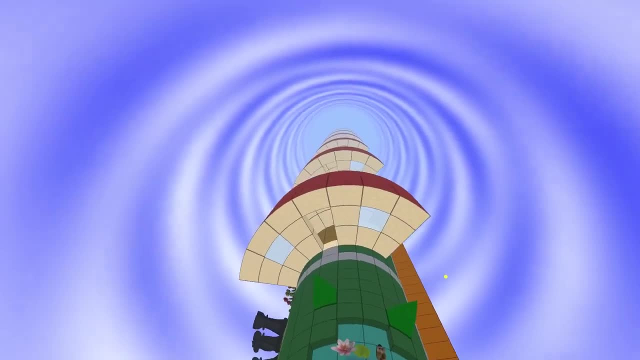 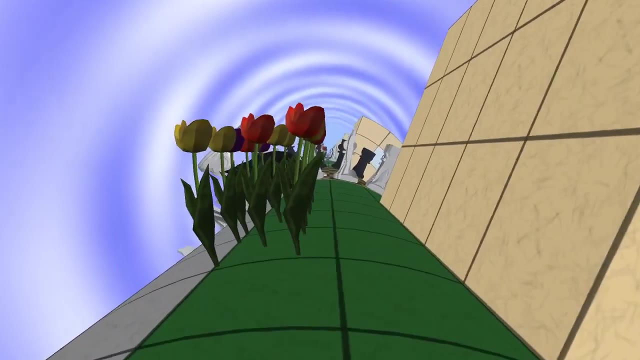 but also vertically. Can we bend and wrap both dimensions at once? Some of you probably thought of taking both ends of a cylinder and connecting them in a donut-like shape, More professionally, a torus. Well, that's a good idea. I hope you liked this video. If you liked it, don't forget to like, comment and subscribe to our channel. See you in the next one. Bye. 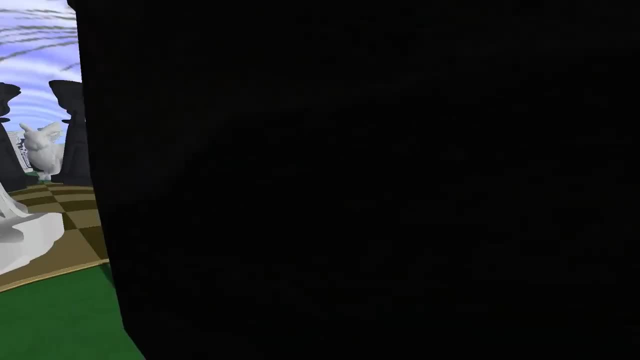 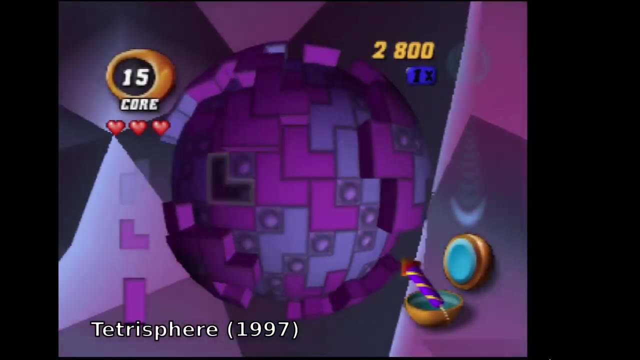 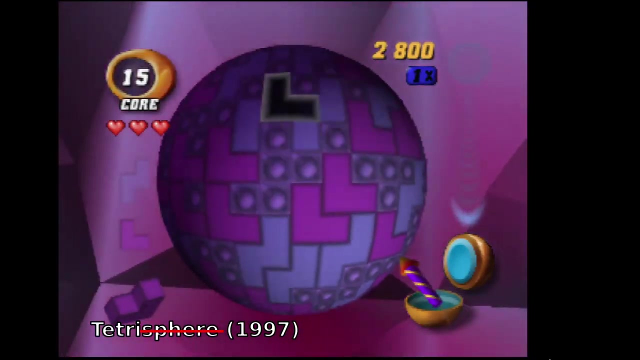 Well, that's a nice idea. Keep that in mind, But for now, we want something different, Something that you might have seen in video games. What is that? Is it a sphere? No, it is not. See, it is tiled with squares By Euler's polyhedron formula. 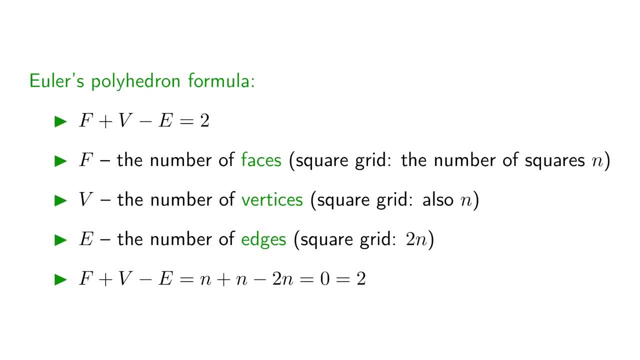 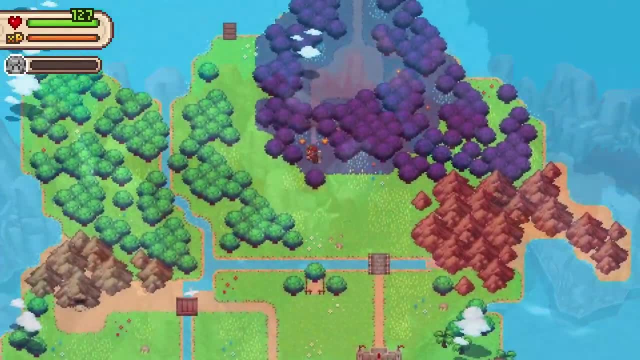 we can prove that it is not actually possible to tile a sphere with squares. Here we have the same object, but the square grid is harder to see and it is not really possible to cut it. Now, what do you think? Are you going to complete this wellbeing? Have you done your homework? Please give us the color. 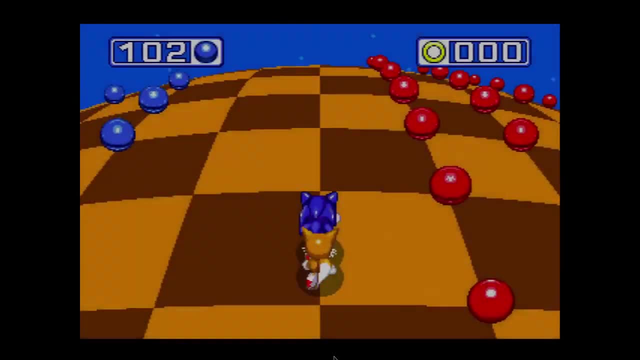 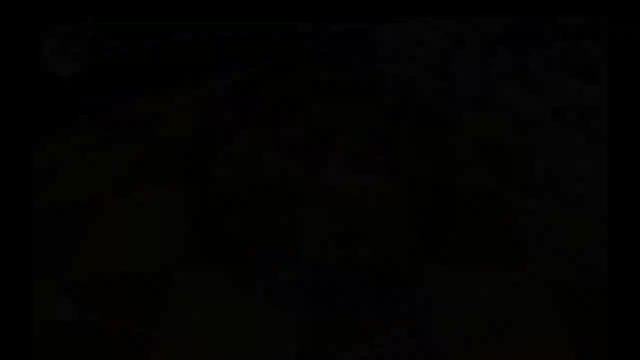 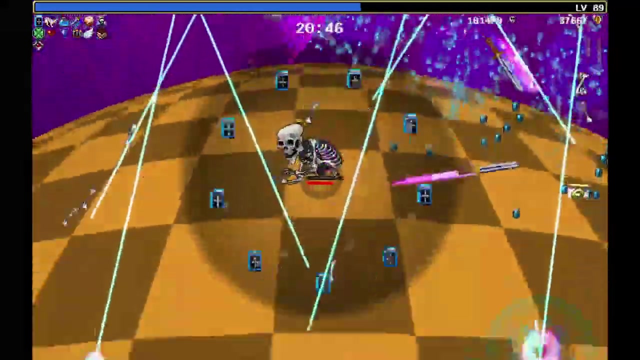 we move to the flat modes in this game, so we see a sphere, but it cannot be a sphere. so what's that, and why something like this? um, these video games must be cheating somehow. oh, here you are. here is the same cheat, but in our small world. 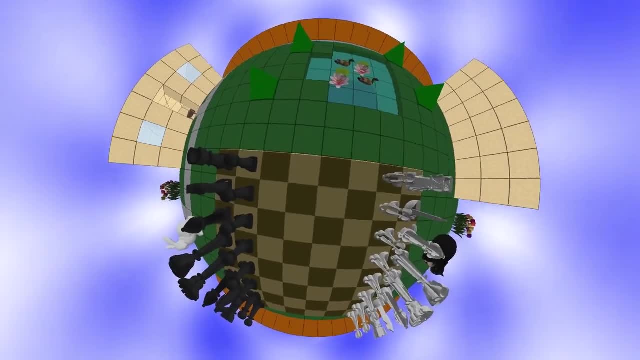 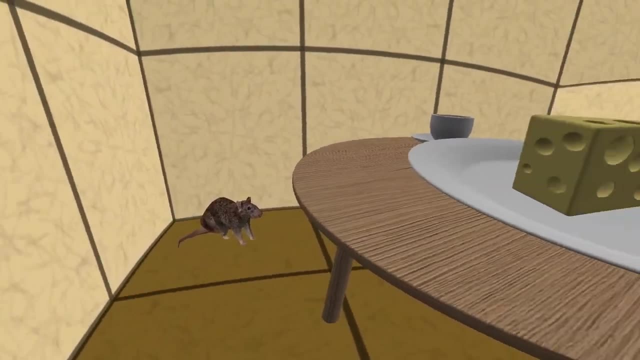 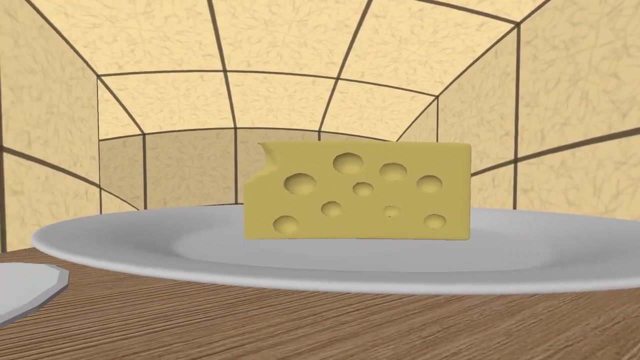 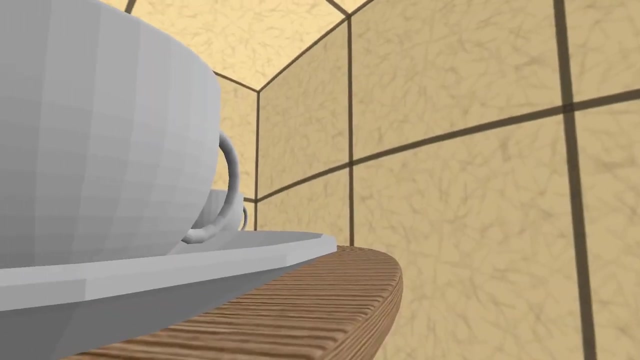 how to explain that. better drink some coffee and grab some cheese while we are thinking about this. hello, mr rat, what a nice cheese with holes, such great holes, holes. how about the hole in our world so we can see what lies below? no, no, no, no, no, no, no. we cannot destroy our beautiful world. the 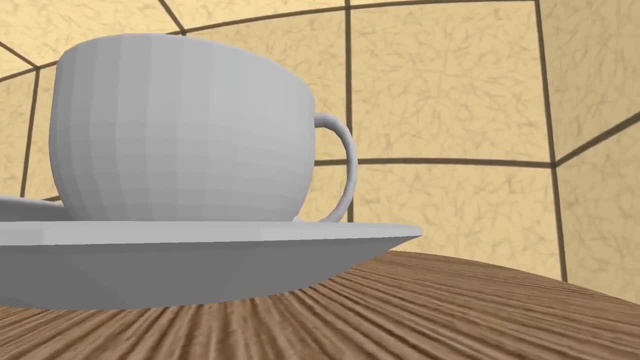 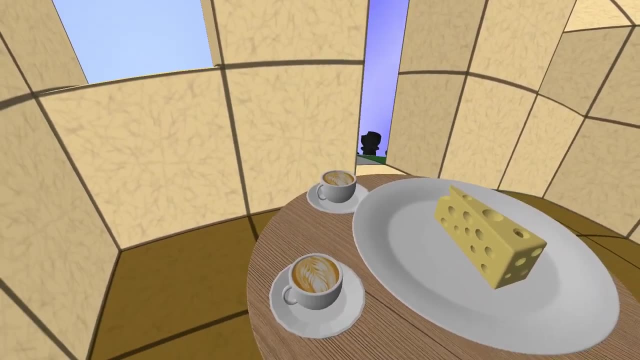 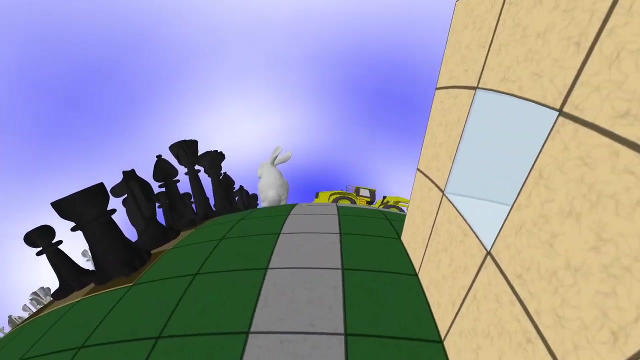 tulips would be lost and the cat and the bunny would be in danger also actually typical games. Games also do not allow you to do so. so no holes, no, no, really no. What's that noise? An evil investor has dug out a big hole in our world. 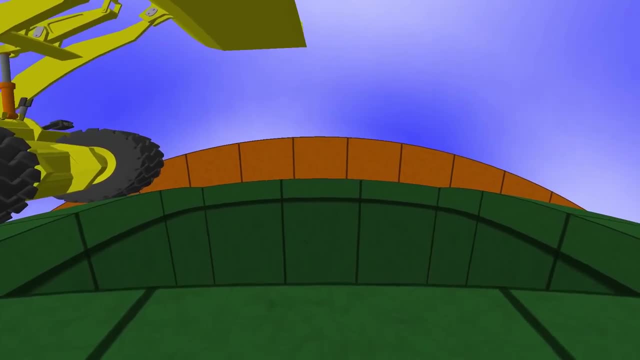 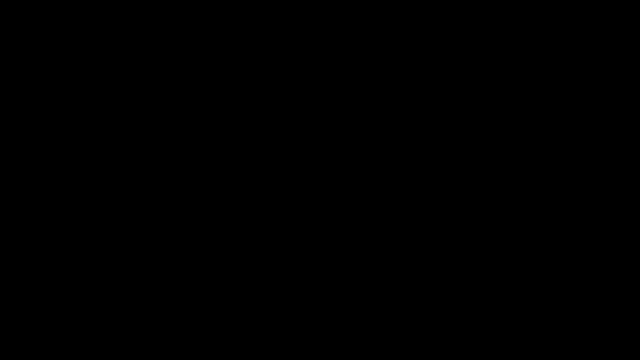 Hmm, it's actually just what we needed. We will use it to move to the other side of our strange object. I suppose you expect it to look like the inside of a sphere, So now we see our fake sphere from the inside. 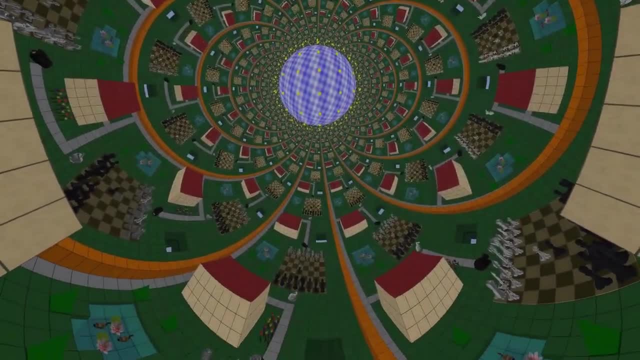 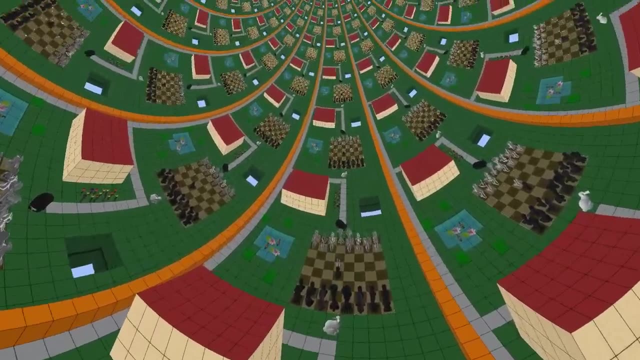 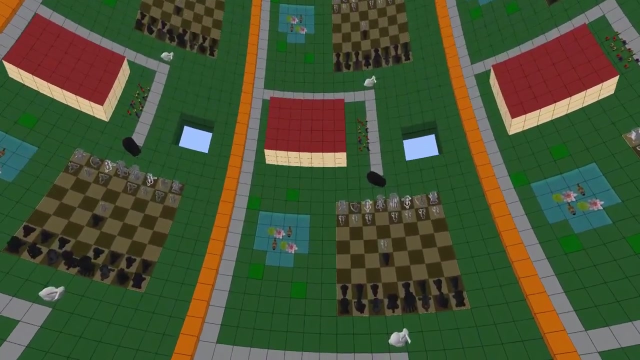 How do you feel about it? Aren't you surprised It was not really tiled with a finite number of squares On the inside. our world also repeats infinitely. Well, probably it's time to name this strange object. It's called a horosphere. 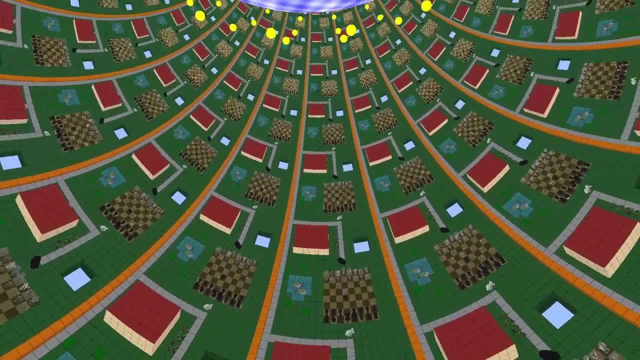 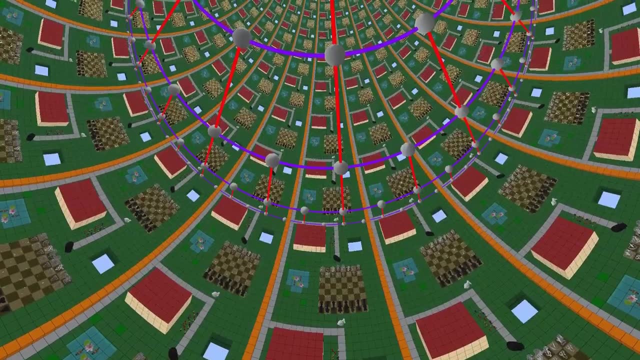 We cannot have a horosphere in the Euclidean geometry. To build it, we actually had to change how it looks. We had to change how the space itself works. For an explanation, look at this structure. You can treat it as a kind of a skeleton of our space. 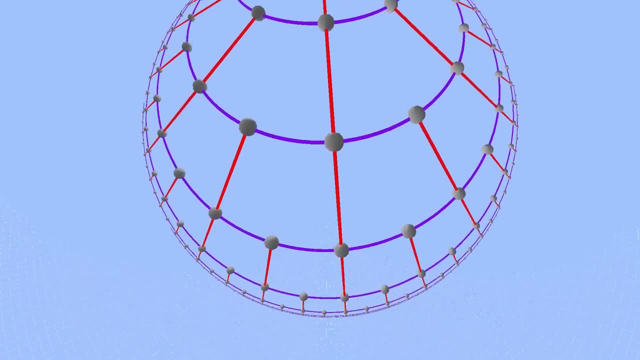 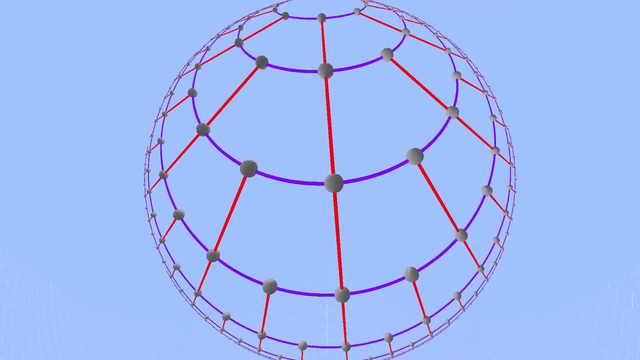 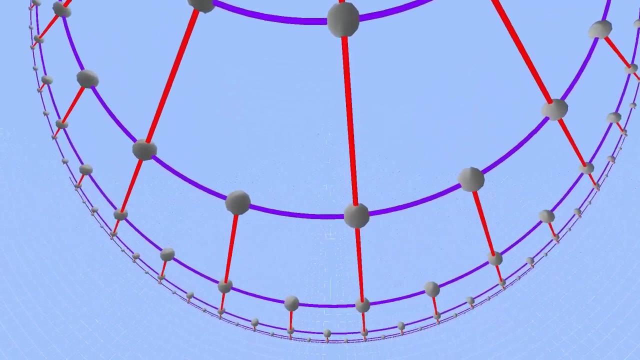 All the red segments are vertical and of the same length, And all the purple segments are horizontal and also of the same length. Note that on every level a horizontal segment corresponds to two segments on the level below. The same doubling would continue infinitely below the ground. 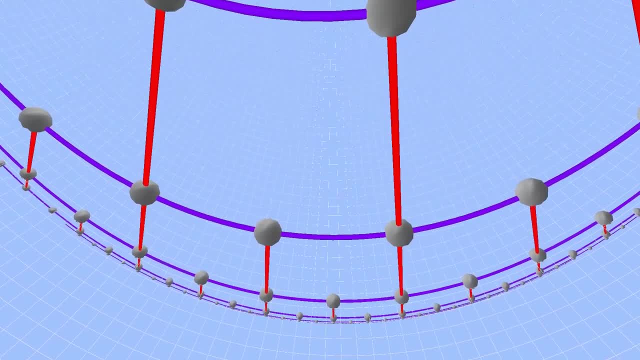 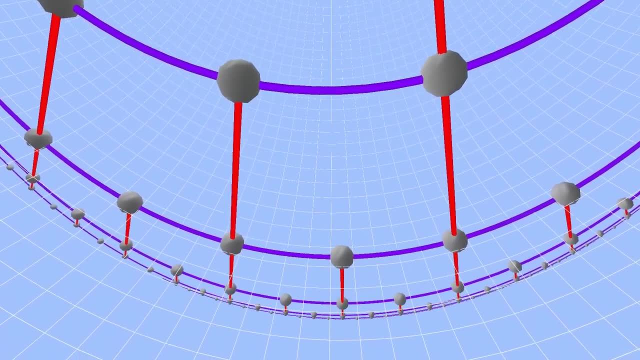 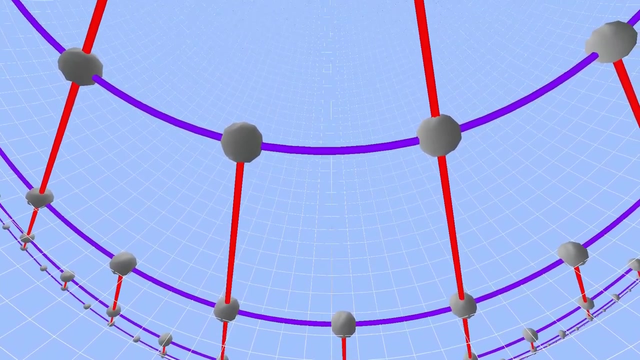 In this world, just like in ours, light always takes the shortest path. Since horizontal distances are shorter, upwards the light will not go horizontally, but curve upwards. That is why those horizontal lines look curved. I said we had needed to change the geometry. 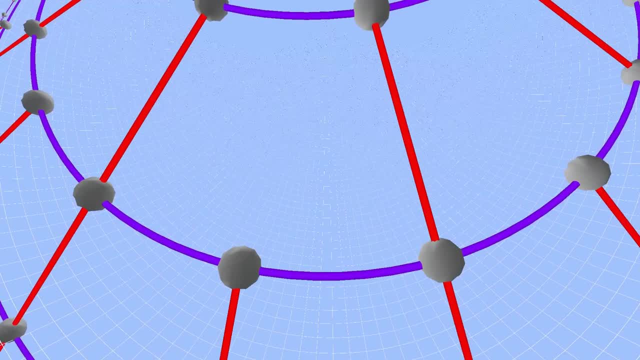 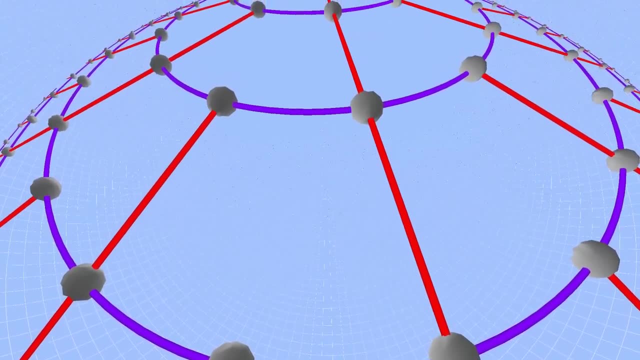 While cylinders could be built in Euclidean geometry, we cannot build horospheres there, simply because there would be not enough space. However, our construction fits perfectly in hyperbolic geometry. Do you remember right-angled pentagons from our previous videos? 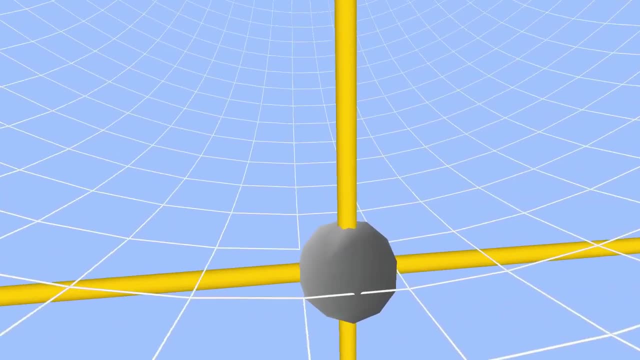 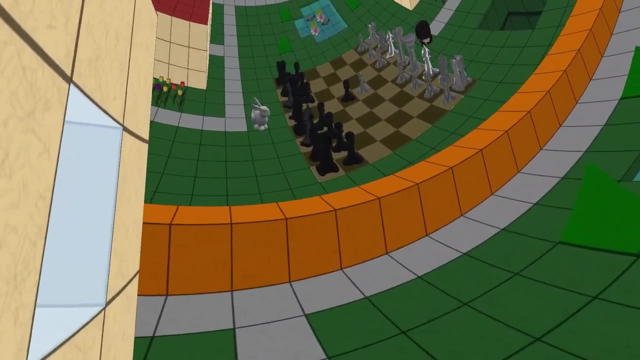 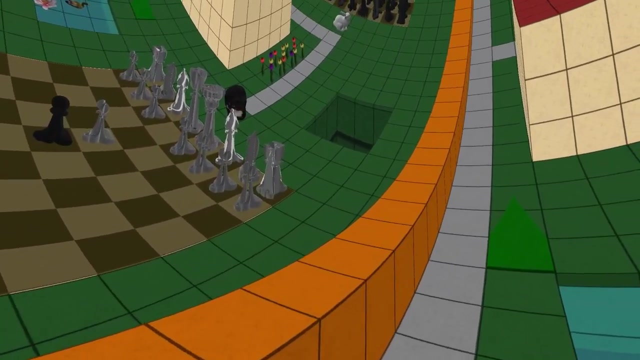 It is the same geometry. So in some sense, the games we have shown were using non-Euclidean geometry. Why aren't they advertised? so, On one hand, this has no practical relevance to the actual gameplay, contrary to an actual non-Euclidean game such as Hyper Rogue. 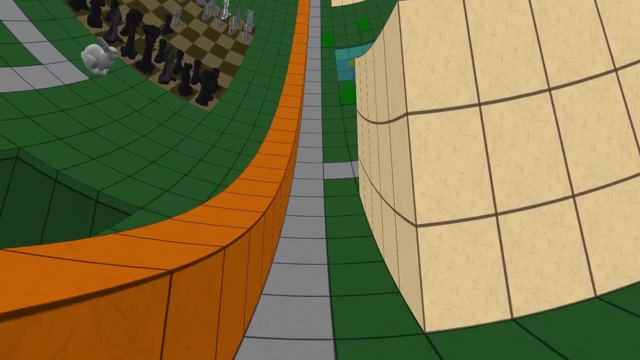 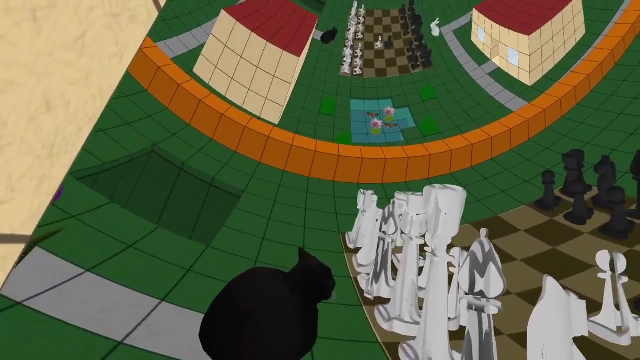 Well, at least if it is done on the ground, If it is done on the outside of the horosphere, When done on the inside, it could be an interesting setting for a first-person shooter, for example, Or at least I think so. 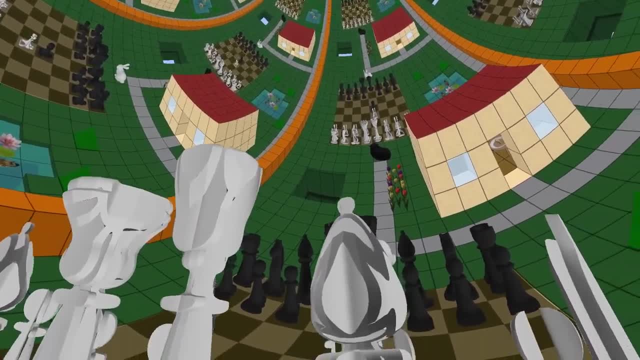 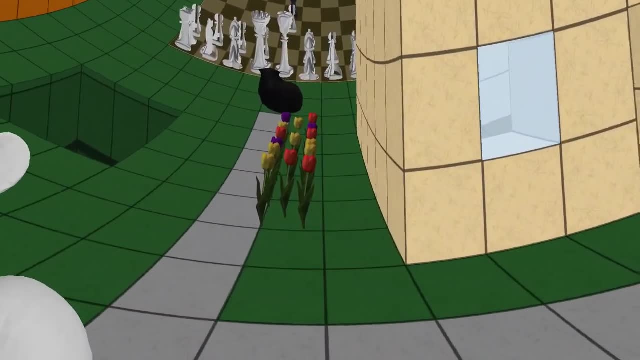 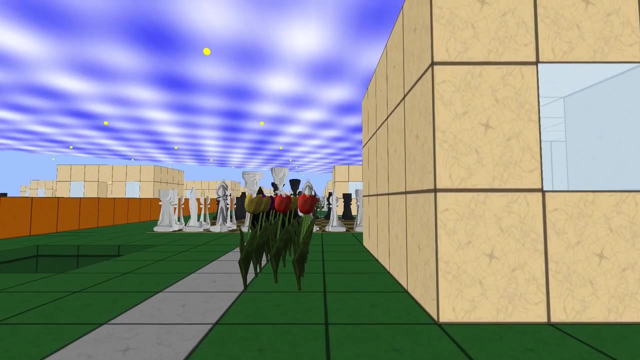 On the other hand, the same visual effect could be obtained using the stereographic projection, which I suppose is how most game devs think about it. These were the things that do appear in games, At least in some sense, But if you want something more exotic, 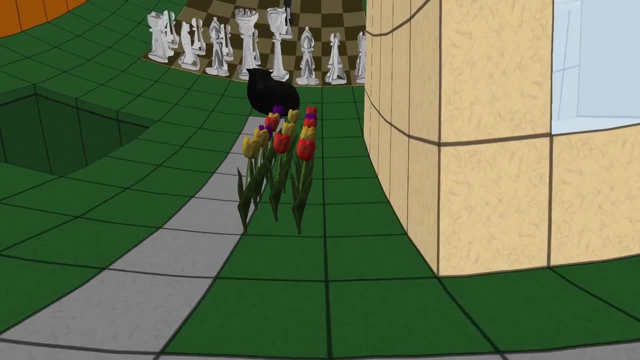 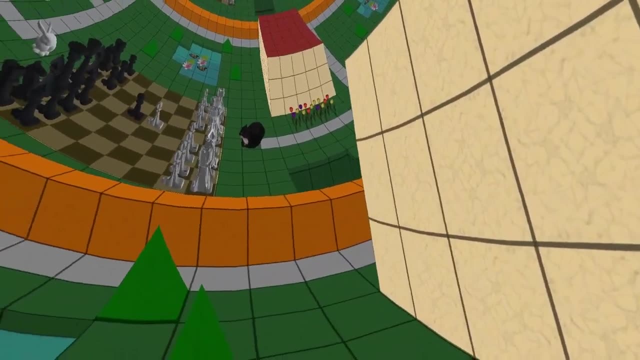 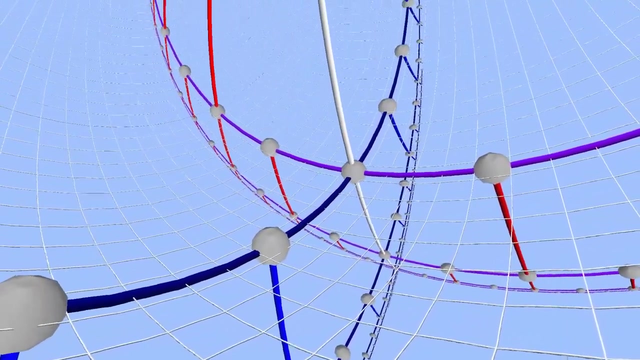 there are more possibilities In our horospherical construction. each vertical level doubles distances in both X and Y coordinates. Let's change that Here. each vertical level doubles distances in X, but in Y the distances are tripled As a result when we move the camera away. 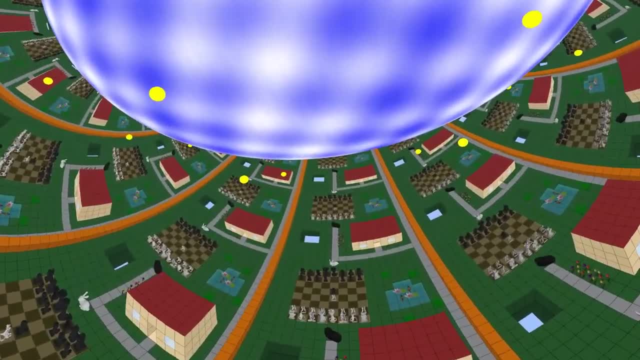 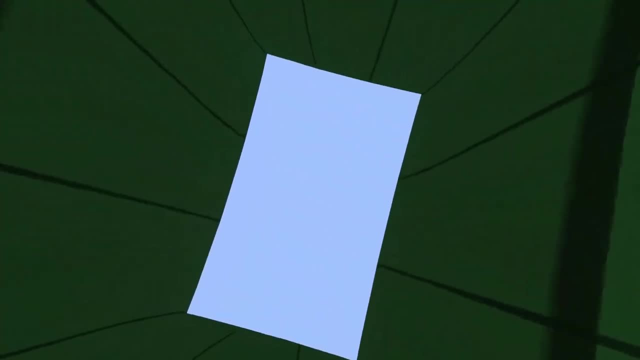 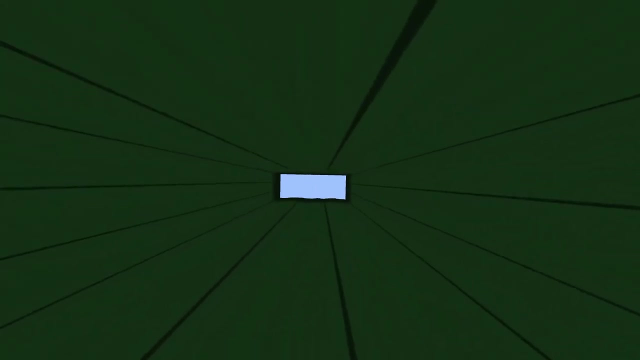 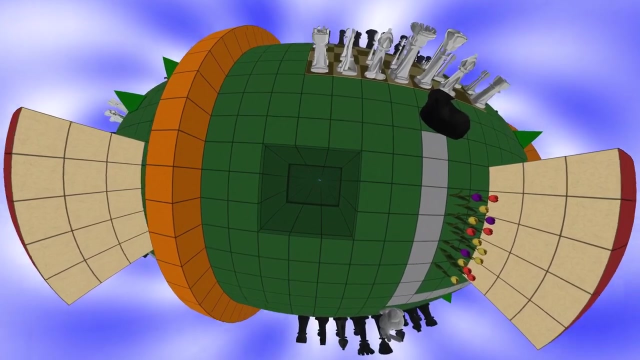 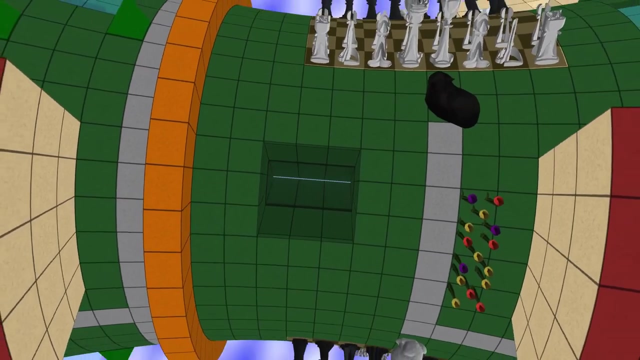 the squares no longer look like squares. Also, the horizontal levels look more like ellipsoids. Such effects are typical to anisotropic geometries. To see those effects more clearly, we will come back to the surface. Follow me. Here is another strange world. 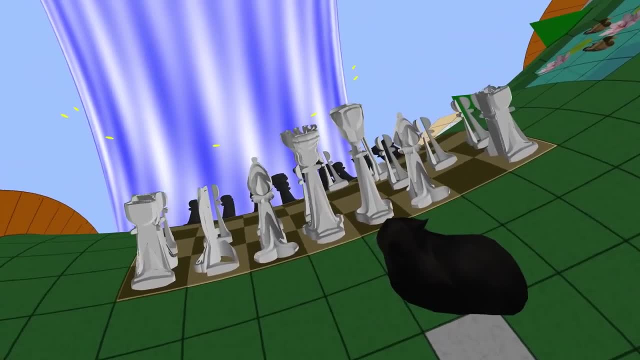 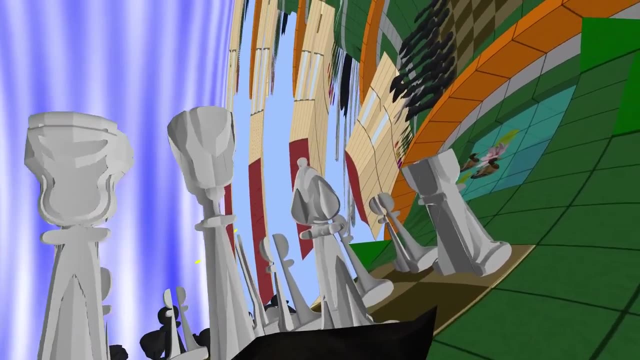 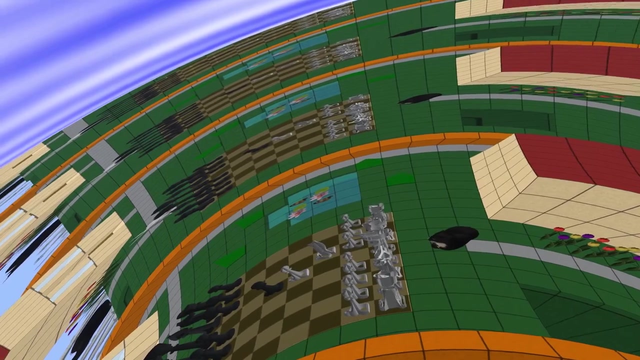 This time, each vertical level doubles the distances in X, but halves the distances in Y. Now the light rays in the X direction curve upwards, while the rays in the Y direction curve downwards. As a result, the effect looks a bit like a torus. 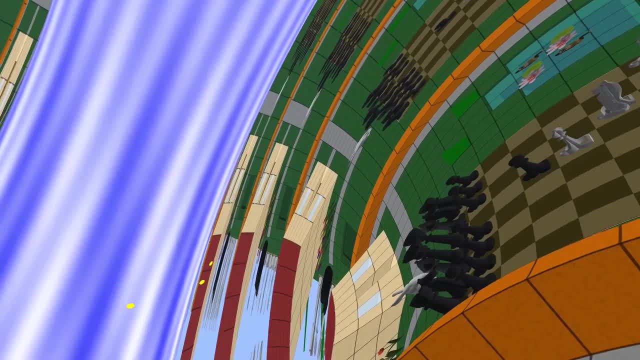 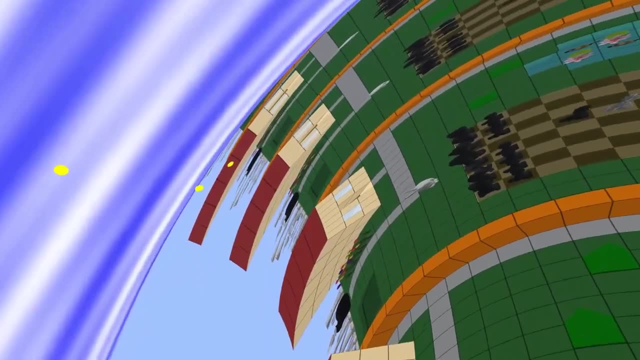 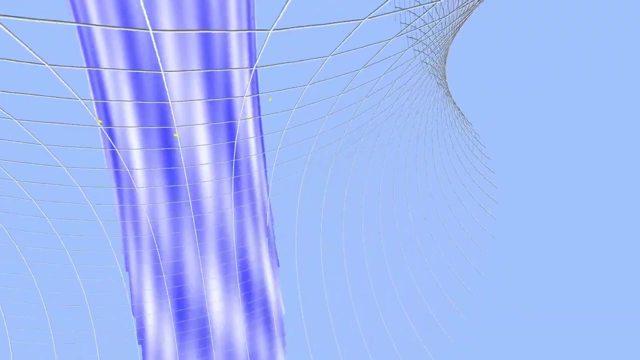 This is the solved geometry, which you might have already seen in our portals video. Let's fly in a straight line for a while. As you can see, the straight lines, or geodesics, in Solve, are quite complicated. Do you see why the shortest paths in Solve behave this way? 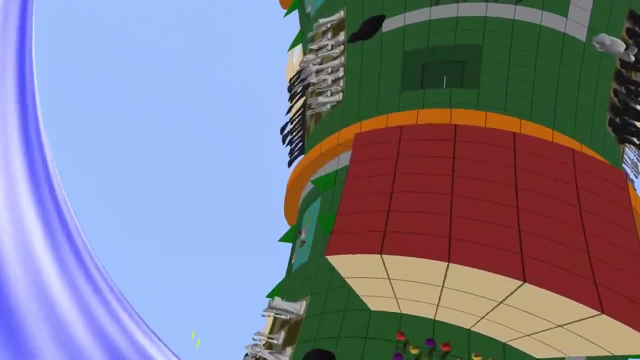 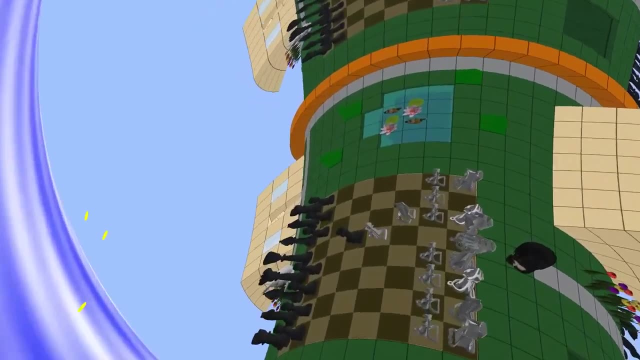 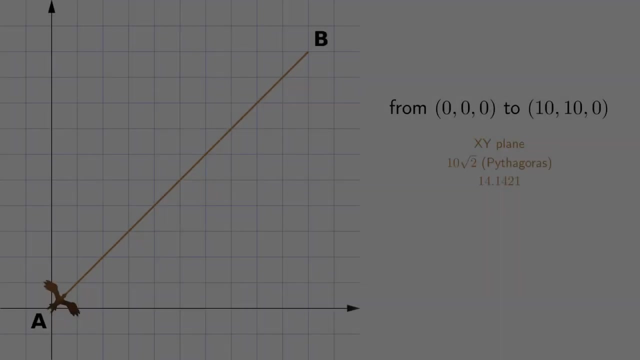 We will explain it in a moment, but if you want to think about it by yourself, please feel free to pause the video. Imagine you want to go from the point A to the point B. Of course we could reach this point without leaving the plane.